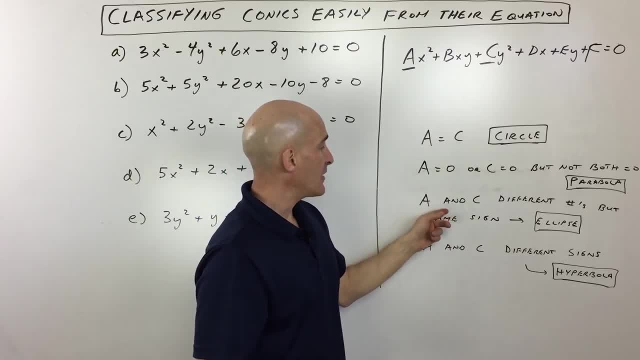 y squared term, then you know it's a parabola. And then if a and c are different numbers but they have the same sign, meaning that they're both positive or they're both negative. so you have like a positive- x squared- and a positive- y squared, or a negative. 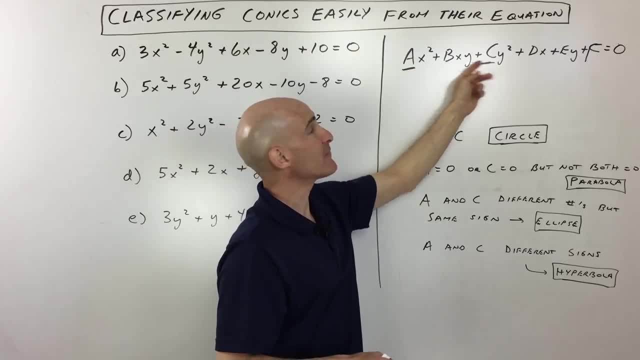 x squared and a negative y squared. But if these numbers are different, then it's an ellipse. And then the last one is that if a and c are different signs, meaning if this is a positive and this is a negative, like you have a positive x squared and negative y squared, or vice versa- 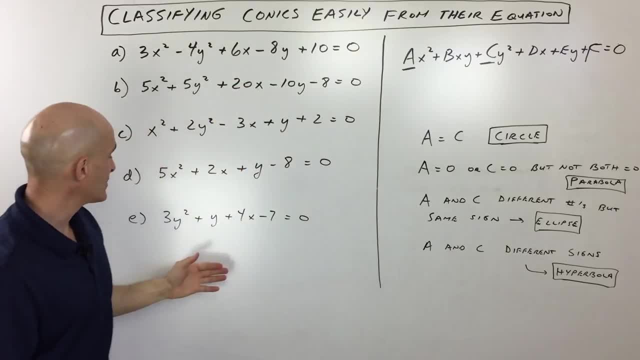 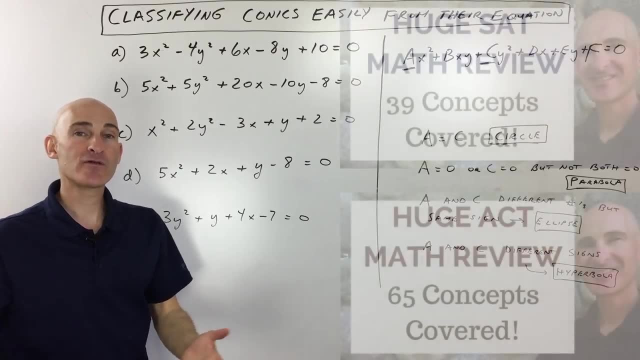 then you know you have a hyperbola. So let's go through some examples here and see if you can identify. you know whether it's a parabola, ellipse, circle, hyperbola, etc. But before I do that, I just want to mention that if you're preparing for the ACT or the SAT, check out my 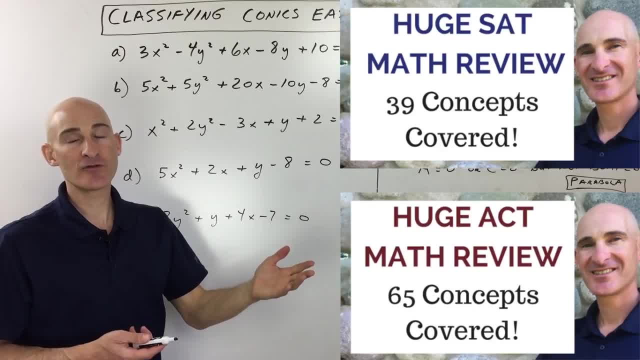 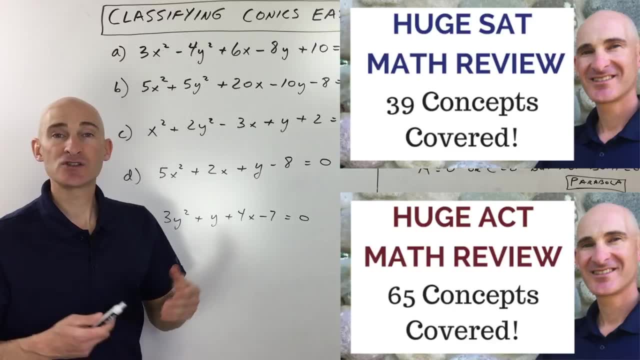 ACT math review video course or my huge SAT math review video course. Those are available for sale through the link below or on my website or on the about page on my YouTube channel. So if you're preparing for those tests and you want to go over some concepts and look at, 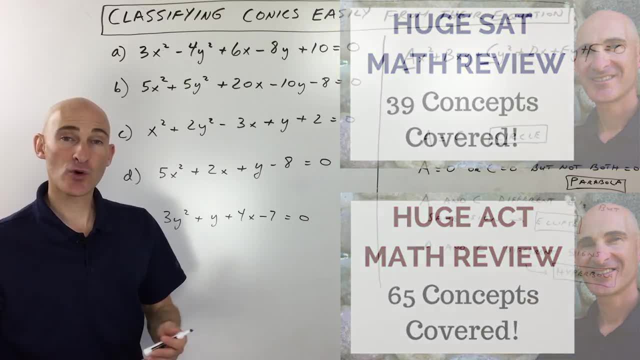 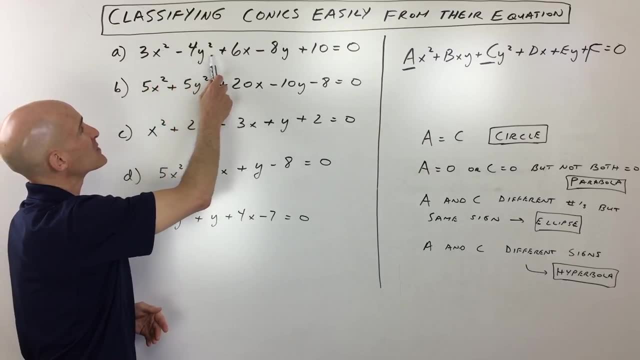 teaching and examples and prepare yourself better for scoring high on that test. definitely check out those video courses, But let's go through these examples here. So we've got the first one: 3x squared minus 4y squared plus 6x minus 8y plus 10 equals 0.. Okay, so what we want to zero in on? 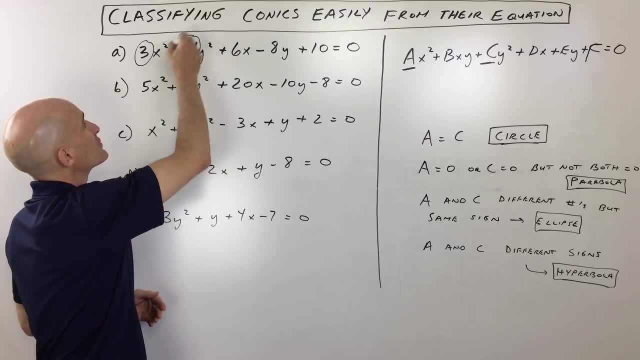 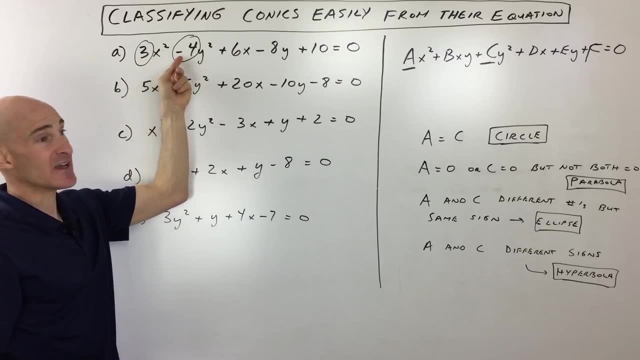 the coefficient in front of the x squared term and the coefficient in front of the y squared term. You can see that there are different numbers and there are also different signs. This is positive, this is negative. So, when there are different signs, a and c, okay, the coefficients in front. 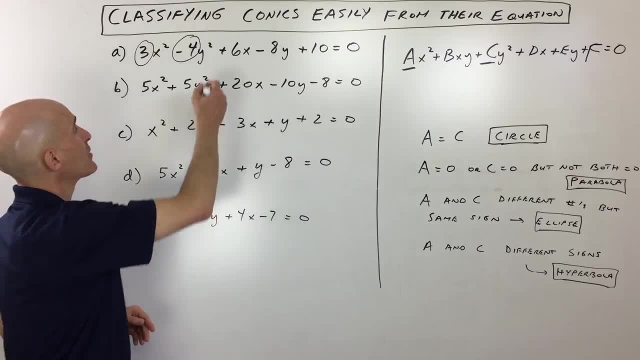 of x squared and y squared. we know that we have a hyperbola, So this one right here, we'll just write h for hyperbola. Okay, the next one. we've got 5x squared plus 5y squared. 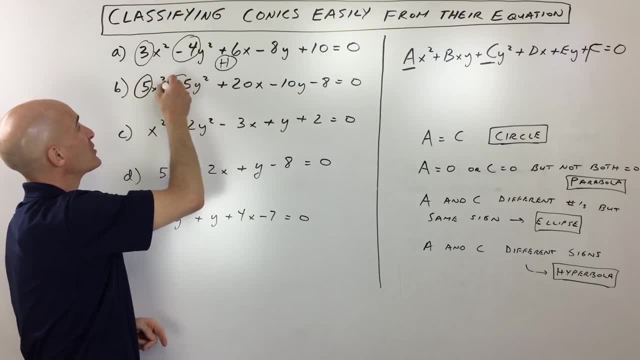 so on and so forth. But again we're trying to zero in on that coefficient in front of the x squared term. Here you can see that they're exactly the same sign, they're exactly the same number. You can see a is equal to c, so we know it's a circle. Okay, and the next one we'll put. 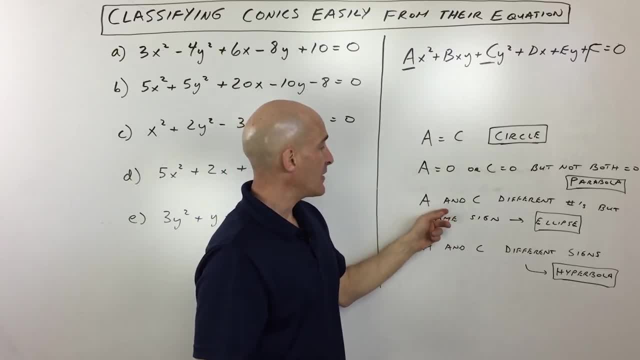 y squared term, then you know it's a parabola. And then if a and c are different numbers, but they have the same sign, meaning that they're both positive or they're both negative, so you have like a positive x squared and a positive y squared or a negative, x squared and a negative y squared. But if these numbers are different, then it's an ellipse. 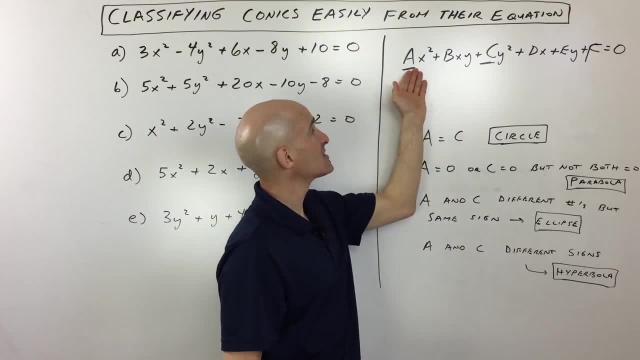 And then the last one is that if a and c are different signs, meaning if this is a positive and this is a negative, like you have a positive x squared and negative y squared, or vice versa, 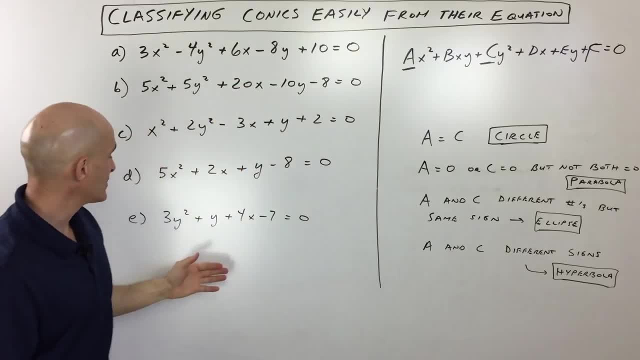 then you know you have a hyperbola. So let's go through some examples here and see if you can identify, you know, whether it's a parabola, ellipse, circle, hyperbola, etc. But before I do 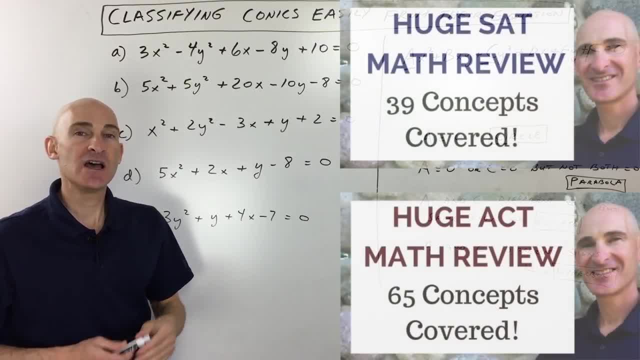 that, I just want to mention that if you're preparing for the ACT or the SAT, check out my 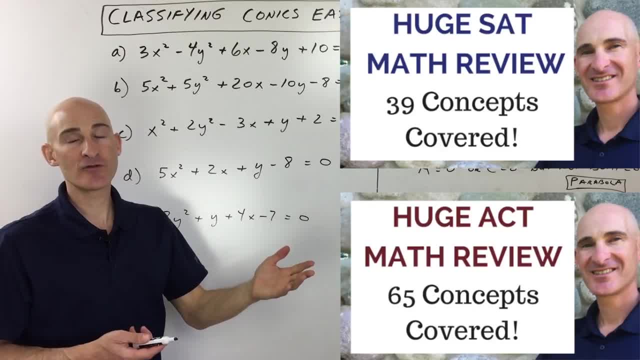 ACT math review video course or my huge SAT math review video course. Those are available for sale through the link below or on my website or on the about page on my YouTube channel. 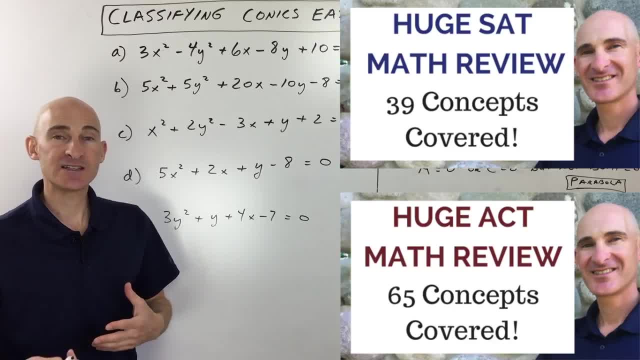 So if you're preparing for those tests and you want to go over some concepts and look at teaching and examples and prepare yourself better for scoring high on that test, definitely check 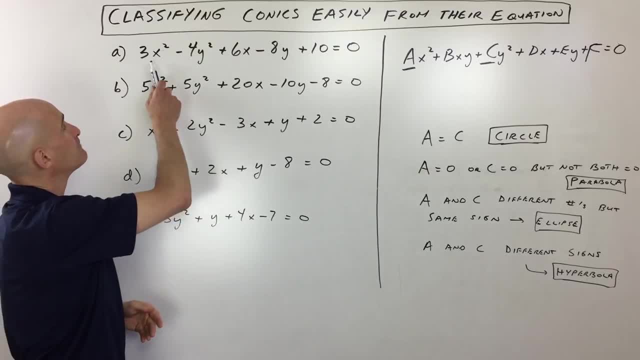 out those video courses. But let's go through these examples here. So we've got the first one, 3x squared minus 4y squared plus 6x minus 8y plus 10 equals 0. Okay, so what we want to zero in on 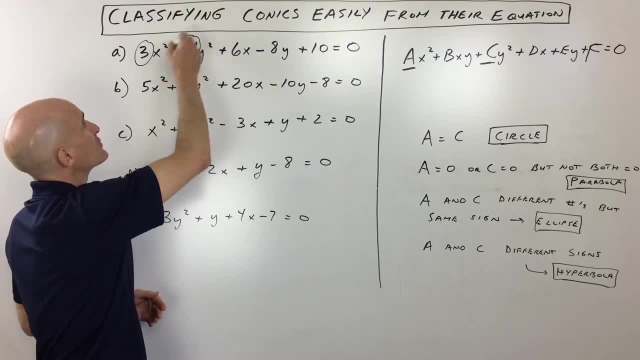 the coefficient in front of the x squared term and the coefficient in front of the y squared term. 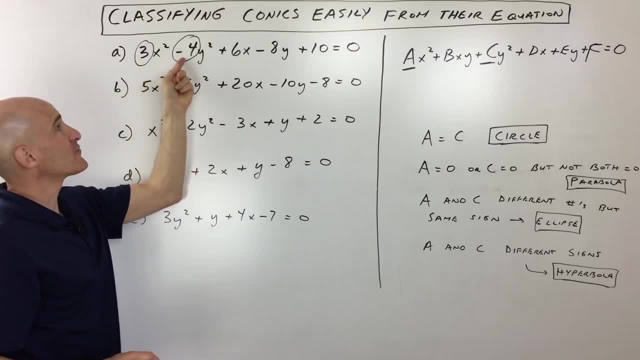 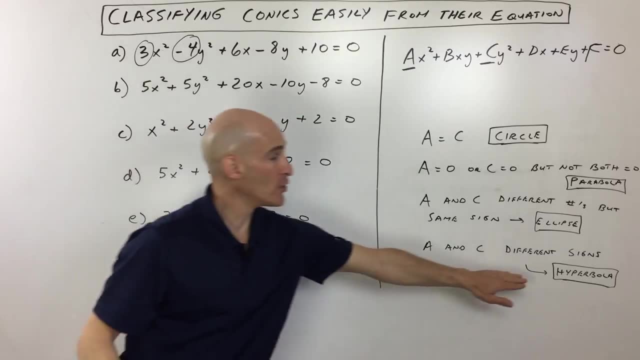 You can see that there are different numbers and there are also different signs. This is positive, this is negative. So when there are different signs, a and c, okay, the coefficients in front of x squared and y squared, we know that we have a hyperbola. So this one right here, 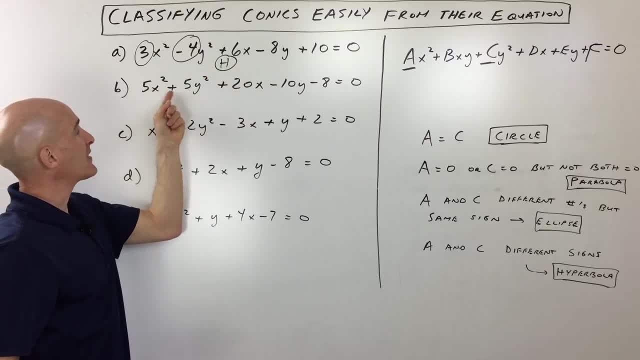 we'll just write h for hyperbola. Okay, the next one, we've got 5x squared plus 5y squared, so on and so forth. But again, we're trying to zero in on that coefficient in front of the x 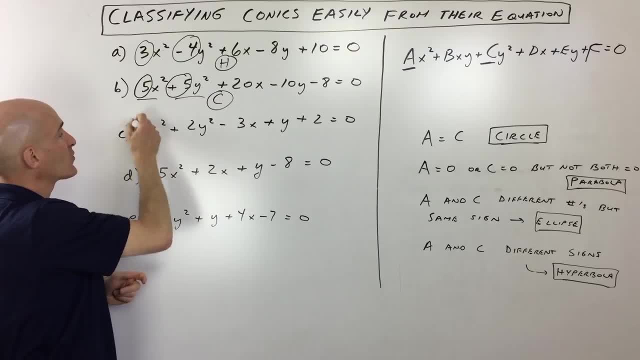 c for circle, for this one, For the next one, you can see: the coefficient in front of the x squared term is 1, the coefficient in front of the y squared term is positive 2.. You can see that they have the same sign, meaning that they're both positive. okay, but they're different numbers. 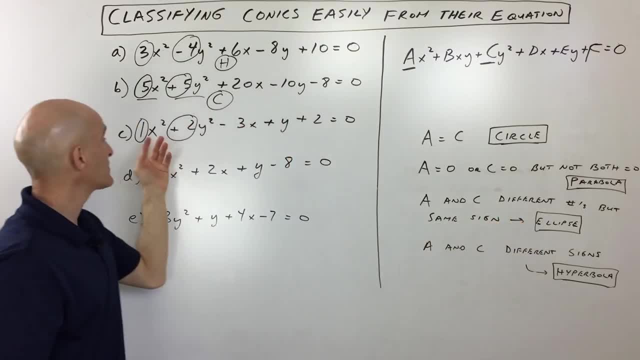 So that means that it's an ellipse, okay. If they were the same sign and the same number, then we'd have a circle. We had the one just above it. So this one's an ellipse, okay. and then this one letter d: 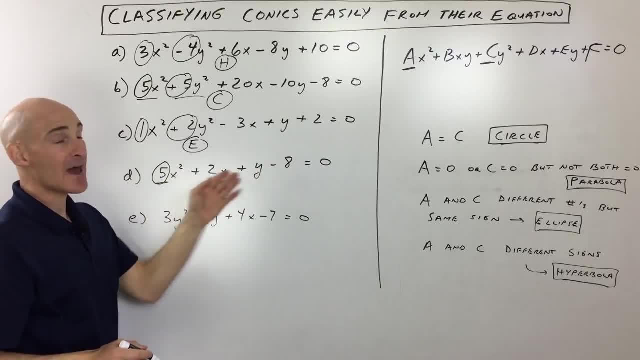 you can see that we have a coefficient in front of our x squared term. There's not a y squared term, so that tells us that this is a parabola. Okay, and then the last one: we've got 3y squared plus. 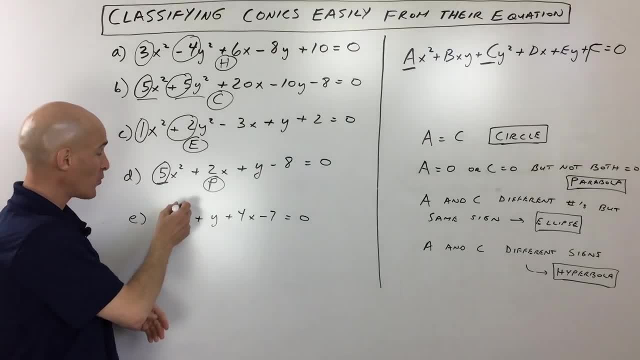 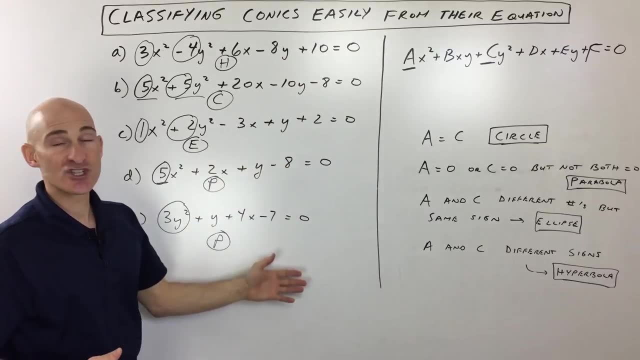 y plus 4x minus 7.. You can see there's not an x squared term here, just a y squared term. So again we have another parabola. So this is a quick way to just identify, when you're given this in the general form like this, whether you have a circle, ellipse. 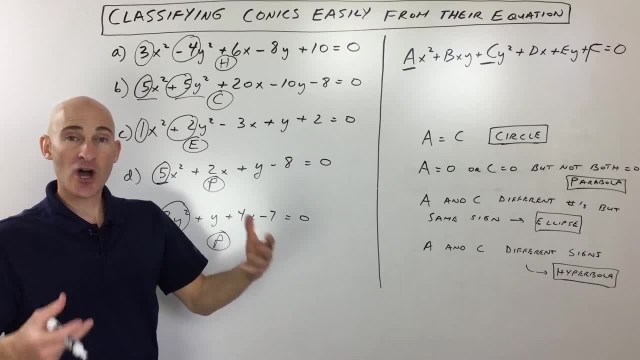 hyperbola parabola. Check out some of the other videos that I did talking about how to write these in the standard form of a circle or ellipse or hyperbola parabola. I have those videos on my YouTube channel, Mario's Math Tutoring. Subscribe to the channel. check out more math tutoring. 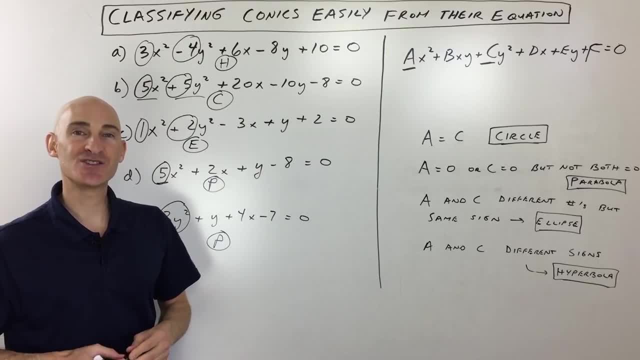 videos over there and I look forward to helping you in the future videos. I'll talk to you soon. 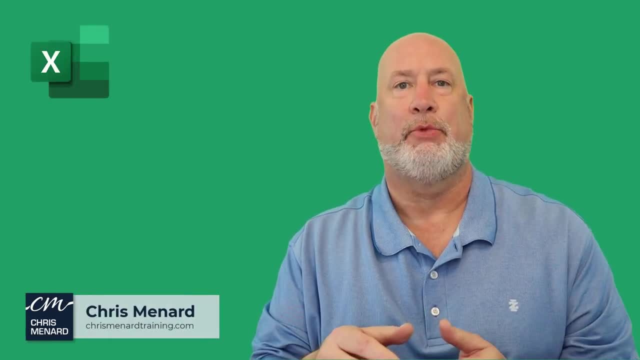 Hello, I'm Chris Menard. In today's Excel video, I'm going to show you how to calculate year-over-year analysis using a pivot table. So this is a great video. in case you're wondering what is year-over-year analysis, It's not always comparing one year to another, even though it's. 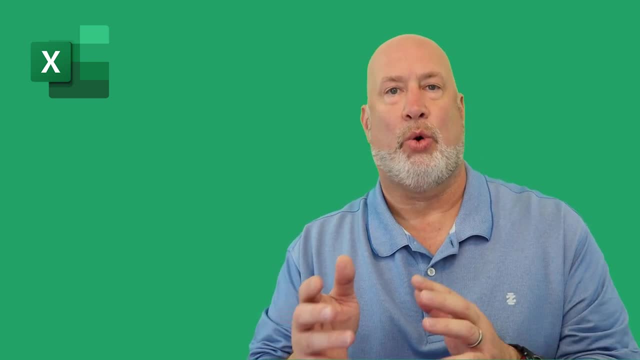 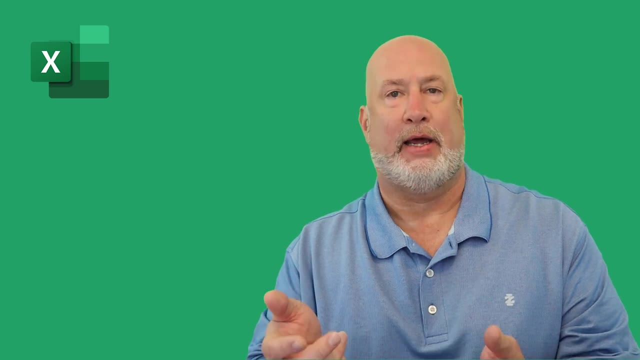 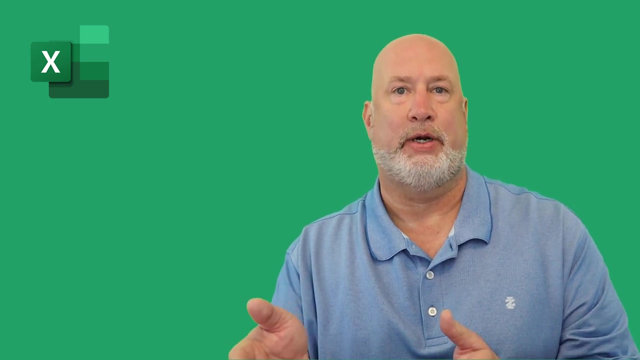 still year-over-year analysis, but it could even be quarters. I want to do the first quarter of 2022 versus the first quarter of 2021. That is called year-over-year analysis. It could also be monthly: August of 2022 versus August of 2021.. And just to show you something real quick: 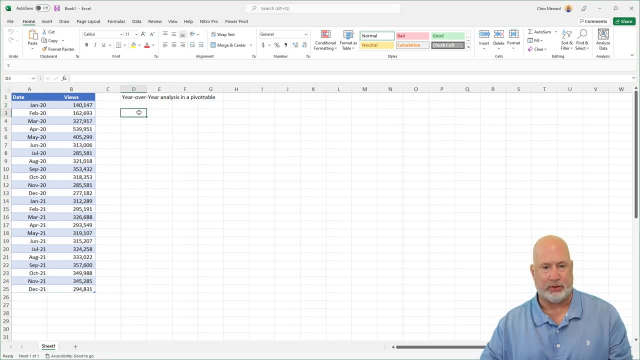 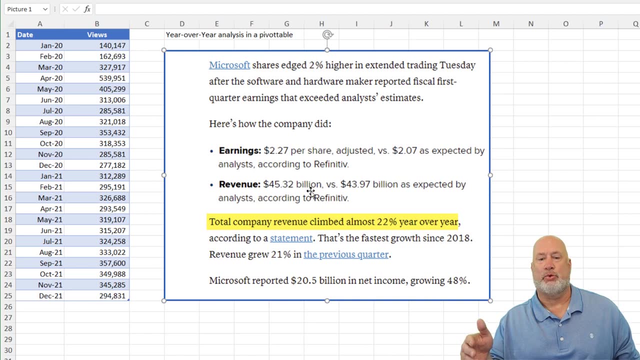 I'm going to throw on this Excel file, a screenshot of Microsoft, and I even highlighted it in yellow to show you this. Total company revenue climbed almost 22% year-over-year, but they're looking at stuff quarterly in this example. So here we go. I've got 24 months of data. I pulled in some views, but this could be revenue.